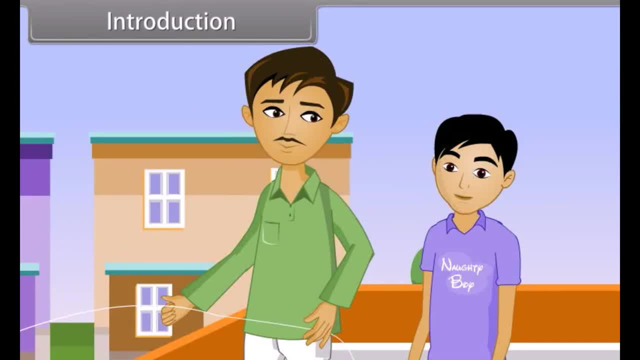 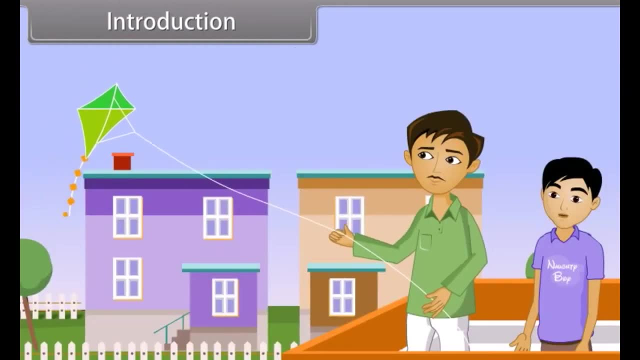 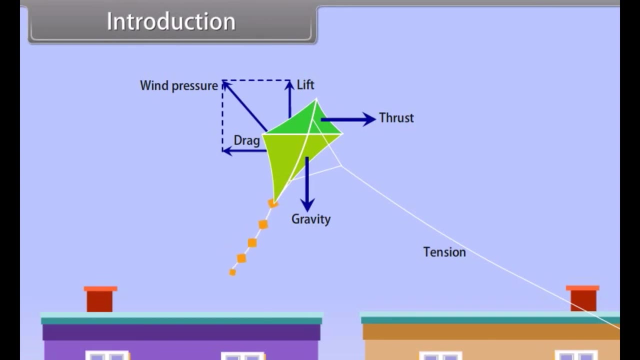 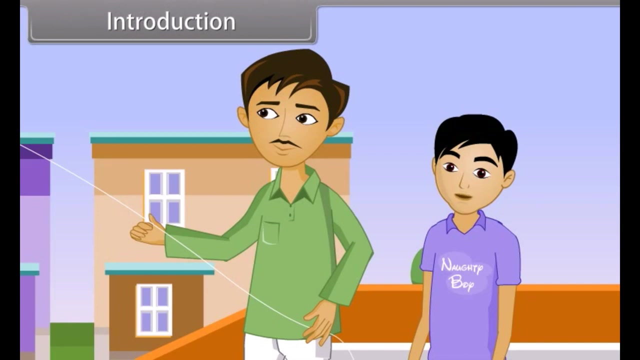 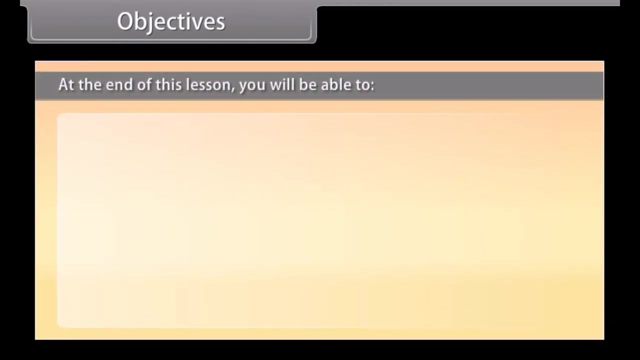 Introduction Objectives. At the end of this lesson you will be able to Differentiate between scalar and vector quantity. Define position vector. Find direction cosines of the position vector. Find additions of vectors. Find components of a vector State section formula for internal and external division. Find dot product of two vectors. 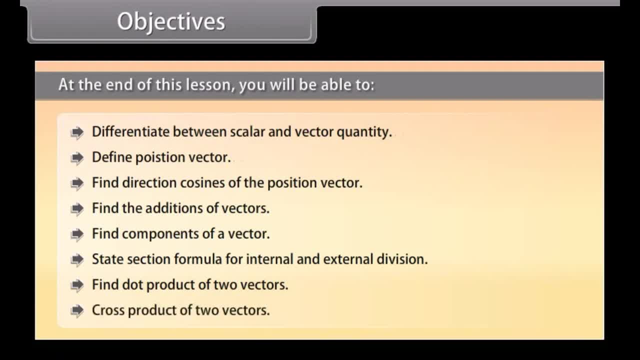 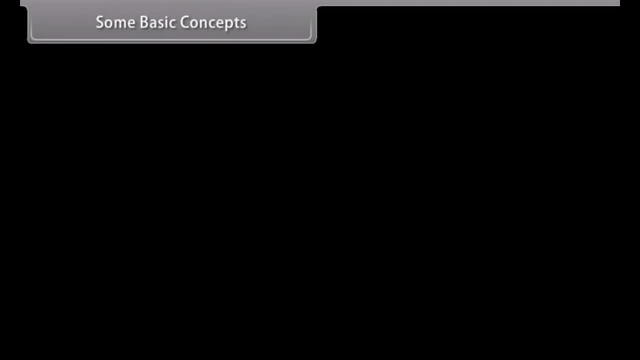 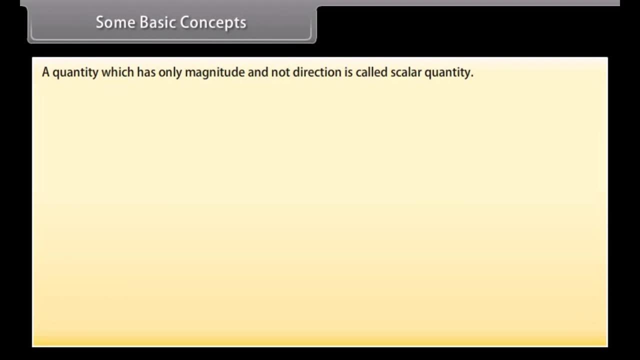 Cross product of two vectors. Some basic concepts: A quantity which has only magnitude and not direction Is called scalar quantity, For example Mass temperature, etc. Let M be a straight line extending indefinitely on both sides. Two points, A and B, on the line AB Are forming the line segment AB. 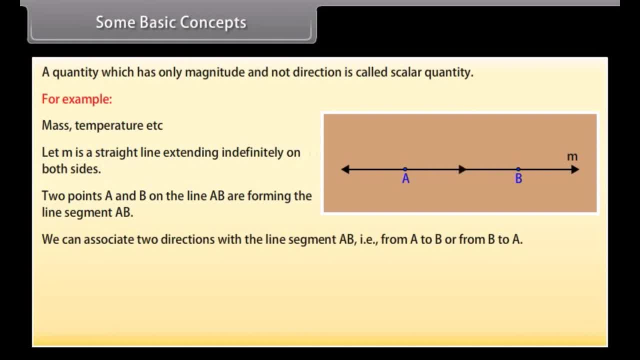 We can associate two directions with the line segment AB, That is, from A to B or from B to A. Thus the line segment AB with fixed direction From A to B or from B to A- Becomes directed line segment AB With A as its initial point And B as its end point or terminal point. 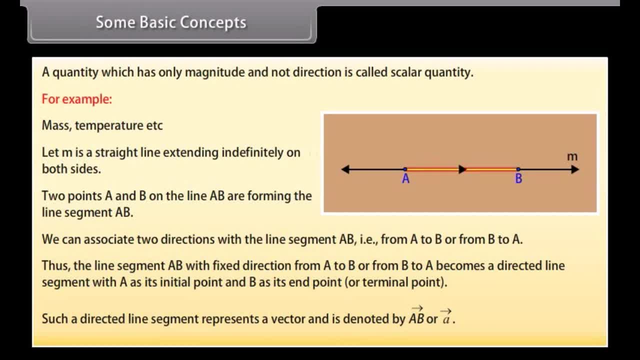 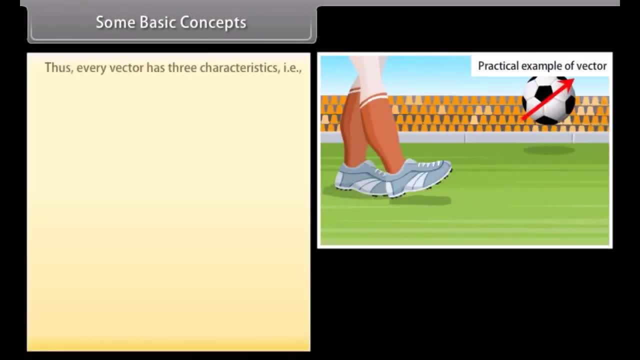 Such a directed line segment represents a vector And is denoted by vector AB or vector A, Practical example of vector. Thus every vector has three characteristics, That is, 1. Magnitude, 2. Direction And 3. Support. Acceleration, velocity, etc. are the three characteristics of a line segment. 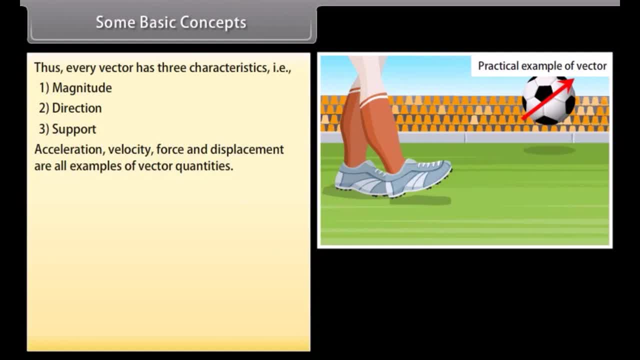 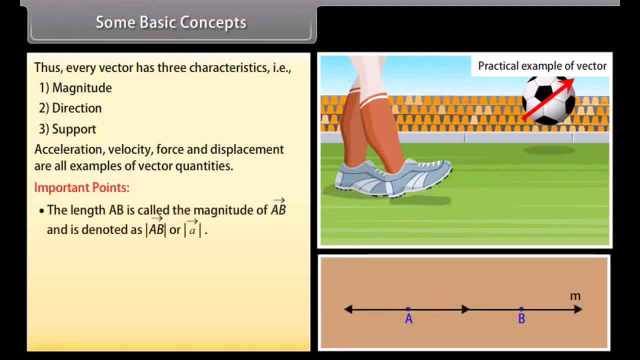 Acceleration, velocity, force and displacement Are all examples of vector quantities. Important points: The length AB is called the magnitude of vector AB And is denoted as mode of vector AB or mode of vector A. The direction of vector AB is from A to B, The line M of which the vector is apart. 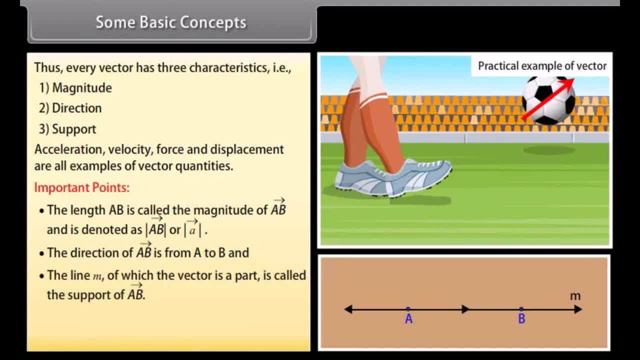 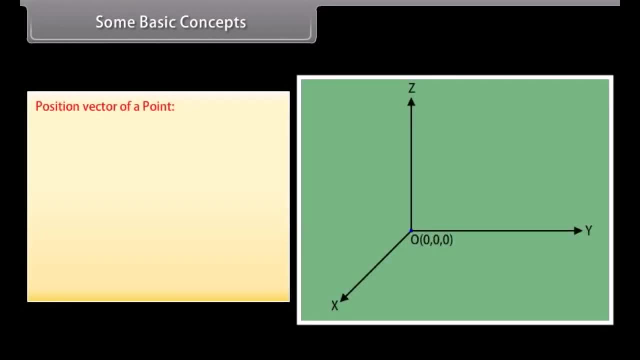 Is called the support of vector AB. Vectors AB and BA have equal magnitude of A to B And same support, But have different directions. Some basic concepts: Position: vector of a point: Let O be a fixed point in space, Called the origin of reference, And B be any point. 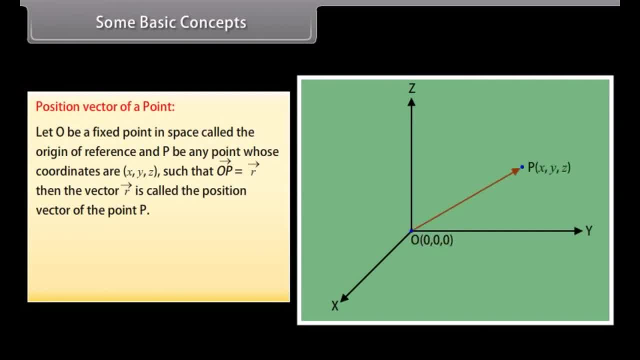 Whose coordinates are X, Y, Z, Such that Vector OP is equal to Vector R, Then the vector R is called The position vector of the point P. The magnitude of the vector R- R is given by Mode of: vector R equals Square root of X square plus Y square plus Z square. 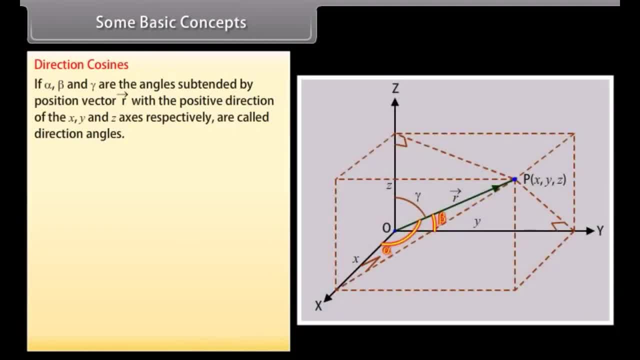 Direction cosines. If alpha, beta and gamma are the angles subtended by position vector R With the positive direction of X, Y and Z axes respectively, Are called direction angles. The cosine value of these angles, That is, cos alpha, cos beta and cos gamma, Are called direction cosines of vector R. 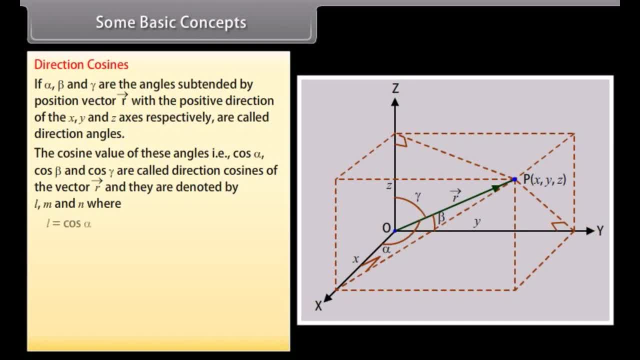 And they are denoted by L, M and N. Where L equals cos alpha, M equals cos beta, N equals cos gamma, Direction cosines are bound such that Minus 1, less than or equal to L, less than or equal to 1, Minus 1 less than or equal to M, less than or equal to 1. 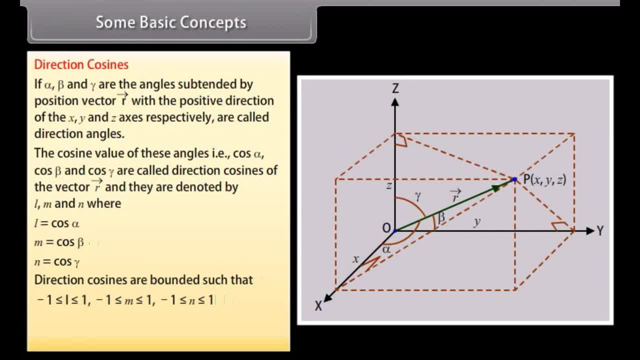 Minus 1, less than or equal to N, less than or equal to 1, Minus 1, less than or equal to 1, And they are connected by the formula: L square plus M square plus N square equals 1. From the figure we can find that 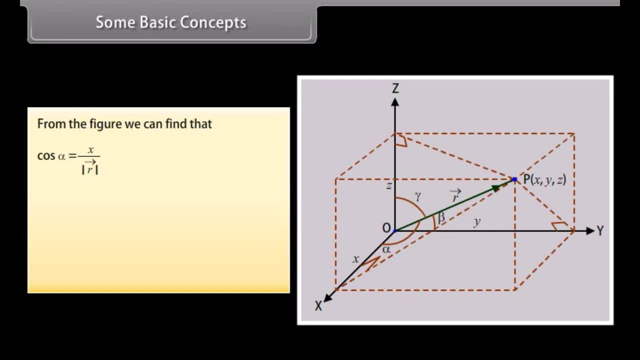 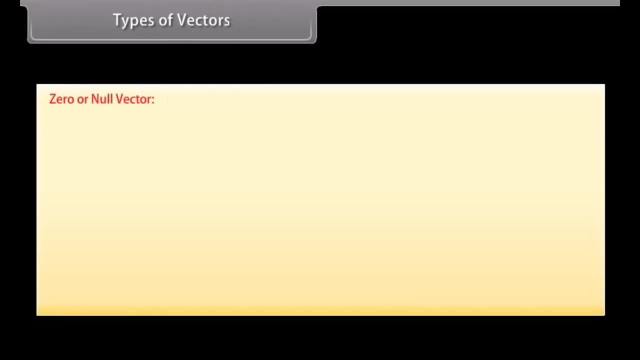 Cos alpha equals X by mode of vector R. Cos beta equals Y by mode of vector R. Cos gamma equals Z by mode of vector R. Types of vectors: Zero or null vector. A vector which has the same initial point and terminal point Is called a zero vector or null vector. 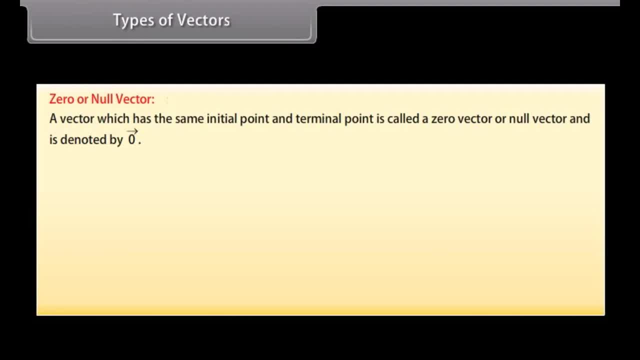 And is denoted by vector. zero Vectors: AA, OO, BB, all are zero vectors. Unit vector: A vector whose magnitude is unity Is called a unit vector For a given vector A. The unit vector in the direction of A Is denoted by cap A And is given by: 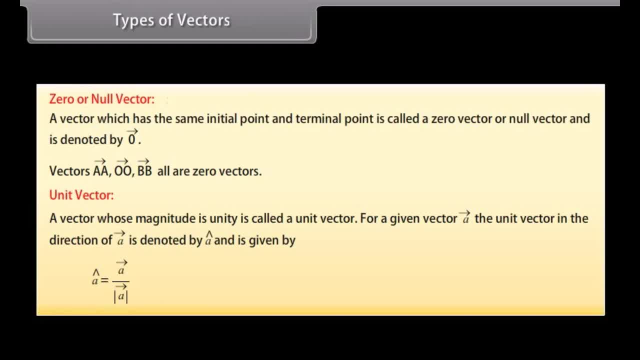 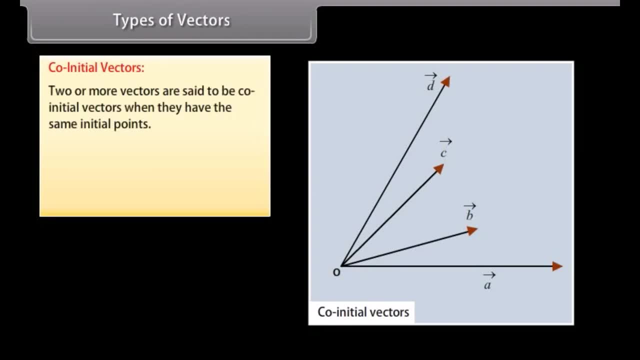 Cap A equals vector A by mode of vector A. Co-initial vectors: Two or more vectors are said to be co-initial vectors When they have the same initial points. For example, Vectors AB, AC, AE and so on are co-initial vectors, Co-linear or parallel vectors. 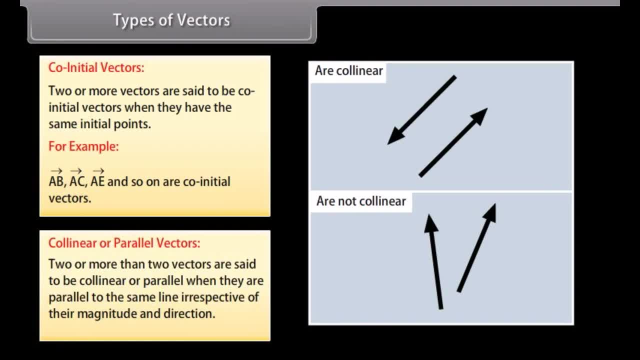 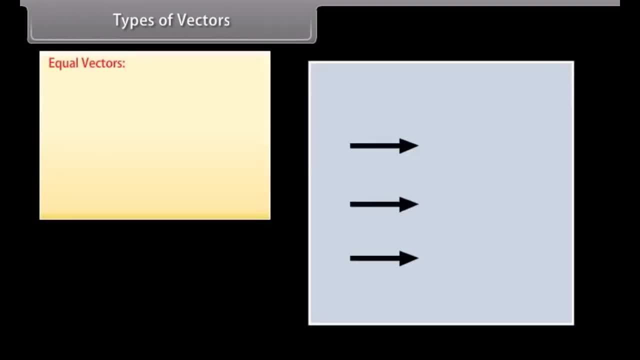 Two or more than two vectors Are said to be co-linear or parallel When they are parallel to the same line, Irrespective of their magnitude and direction. Equal vectors. Two vectors are said to be equal If they have same magnitude, same direction And same or parallel line of support. 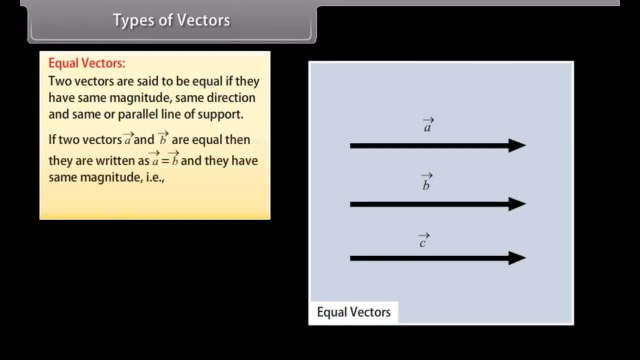 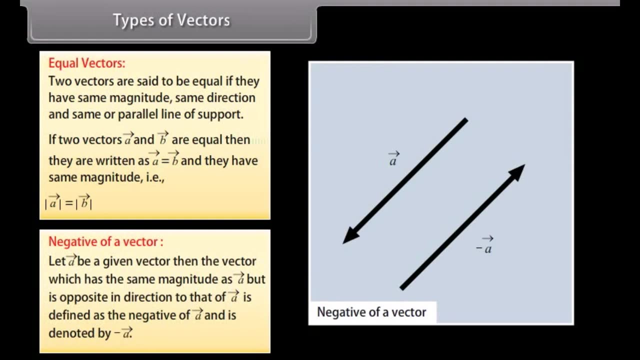 If two vectors, A and B, are equal, Then they are written as vector A equals vector B And they have same magnitude. That is, mode of vector A equals mode of vector B, Negative of a vector. Let vector A be a given vector, Then the vector which has the same magnitude as vector A. 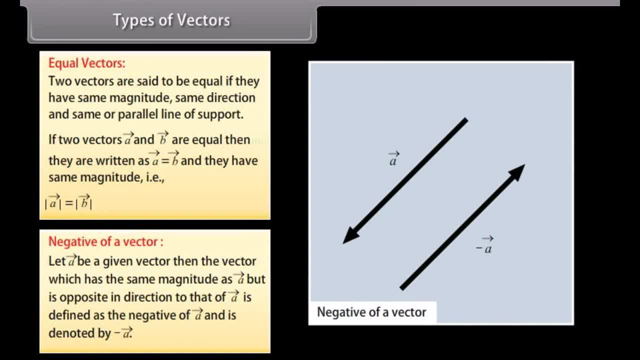 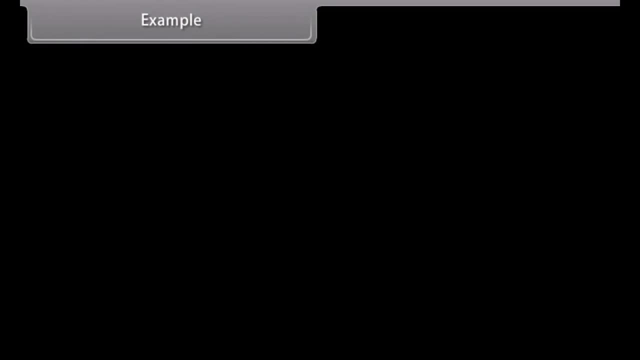 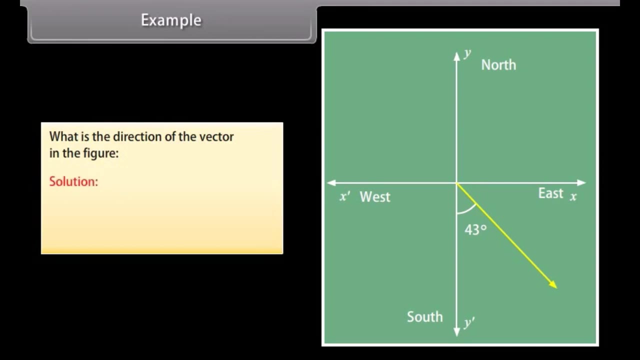 But is opposite in direction to that of vector A, Is defined as the negative of vector A And is denoted by minus vector A. For example, What is the direction of the vector in the figure given below? Solution? The direction of the vector is 43 degree east of south. 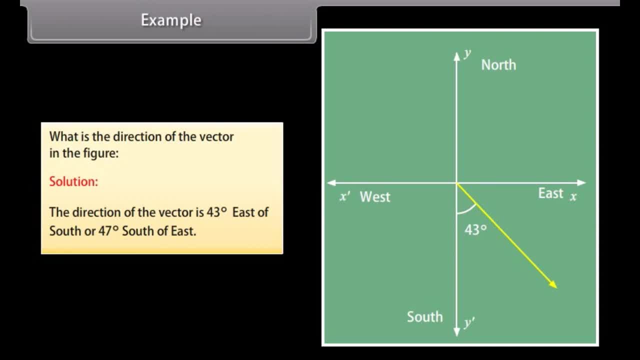 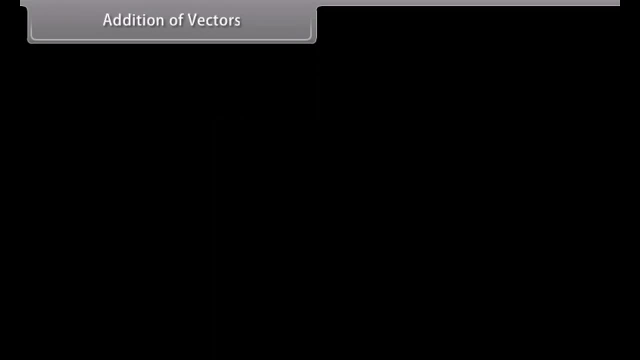 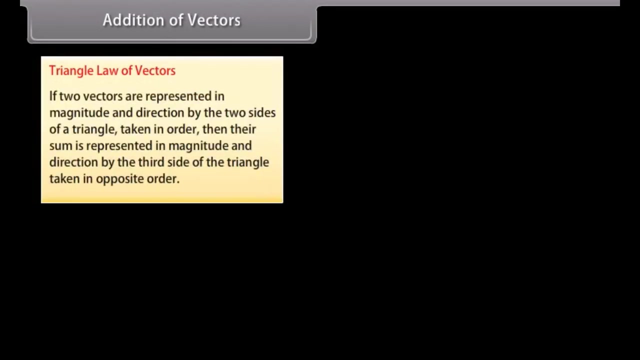 Or 47 degree south of east. Solution: Addition of vectors. Triangle law of vectors. If two vectors are represented in magnitude and direction By the two sides of a triangle, Taken in order, Then their sum is represented in magnitude And direction by the third side of the triangle, Taken in opposite order. 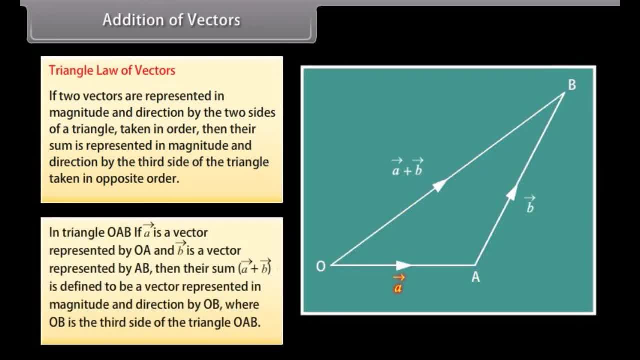 In triangle OAB. If vector A represented by OA and vector B represented by AB, Then their sum, vector A plus vector B, Is defined to be a vector represented in magnitude And direction by OB, Where OB is the third side of the triangle OAB. In vector notation we can write: 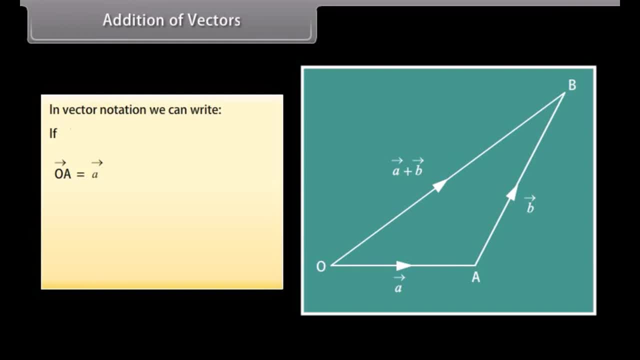 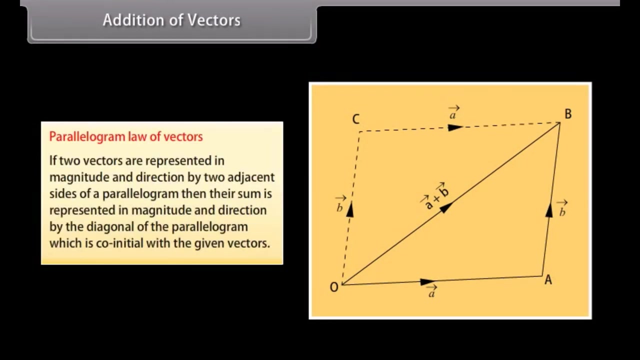 If vector OA equals vector A And vector AB equals vector B, Then vector OB equals Vector A plus vector B, Or vector OA plus vector AB equals vector OB. Parallelogram- law of vectors. If two vectors are represented in magnitude and direction By two adjacent sides of a parallelogram, 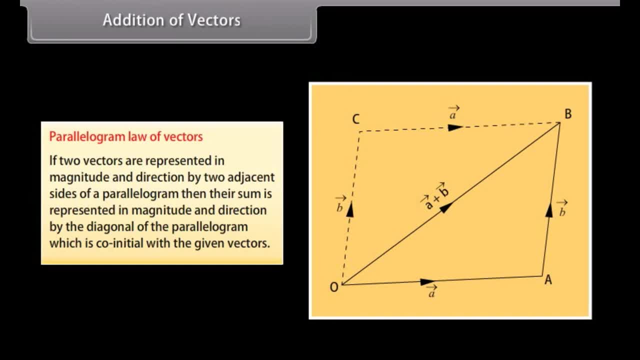 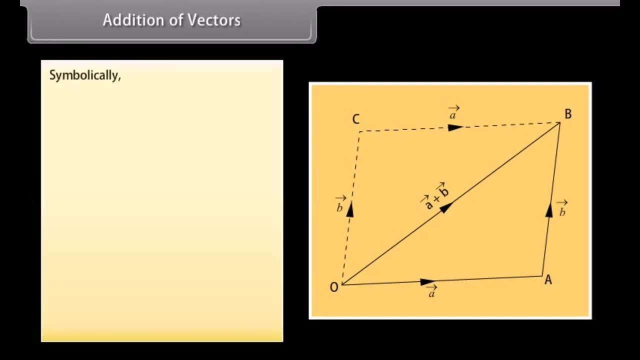 Then their sum is represented in magnitude and direction By the diagonal of the parallelogram Which is co-initial with the given vectors. Symbolically, If vector OA equals vector A, Vector OC equals vector B, Then vector OA plus vector OC equals Vector OA plus vector AB equals. 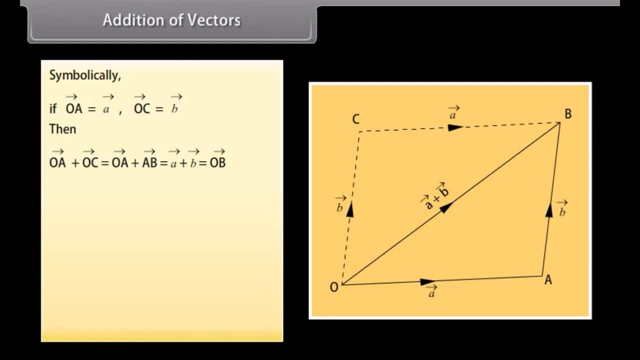 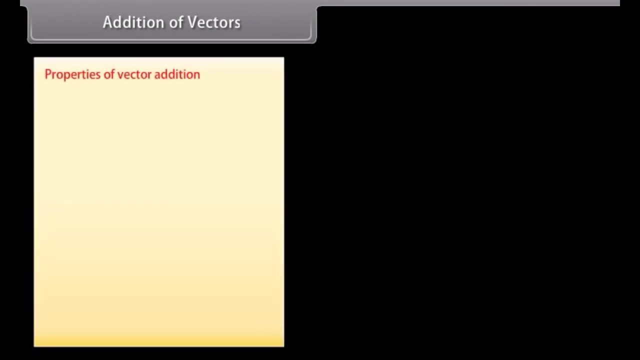 Vector A plus vector B equals vector OB. Therefore vector OC equals vector AB. Also, since vector OC is equal to vector AB, Which equals vector B, Vector CB is equal to vector OA, Which equals vector A. Hence vector OC plus vector CB equals vector OB. Addition of vectors. Properties of vector- addition. 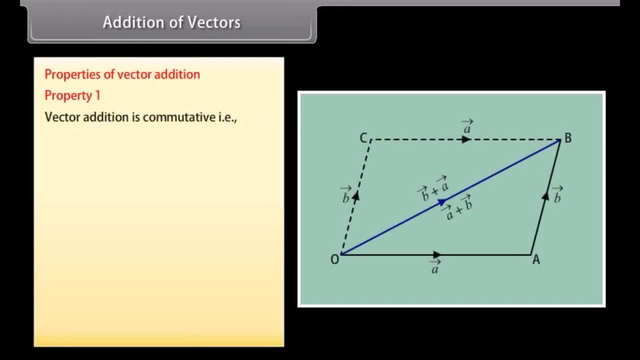 Property 1: Vector addition is commutative, That is, Vector A plus vector B equals vector B plus vector A. Property 2: Vector addition is associative. Here vector R is equal to Vector A plus vector B plus vector C And vector R is equal to Vector A plus vector B plus vector C. 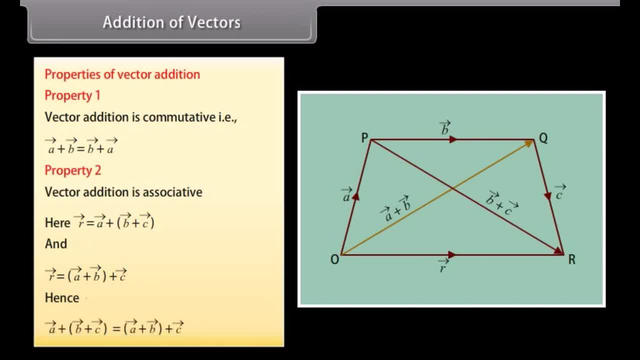 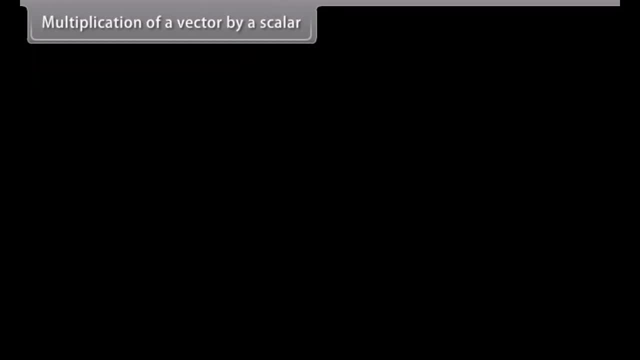 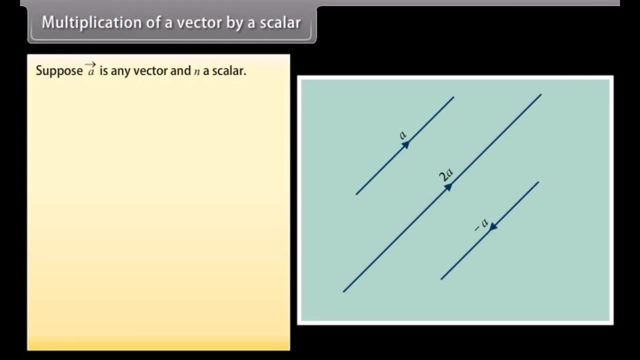 Hence vector A plus vector B plus vector C Is equal to vector A plus vector B plus vector C. Multiplication of a vector by a scalar. Suppose vector A is any vector And N a scalar. By vector N? a we mean A vector whose magnitude is mode of N, mode of vector A. 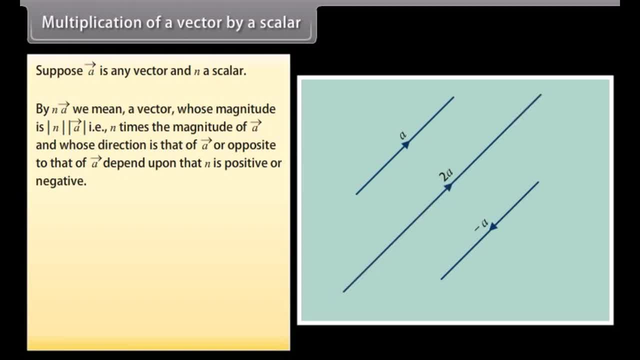 That is N times the magnitude of vector A, And whose direction is that of vector A Or opposite to that of vector A, Depend upon that N is positive or negative. If N is equal to 0, Then 0 vector A is equal to 0. Important results. 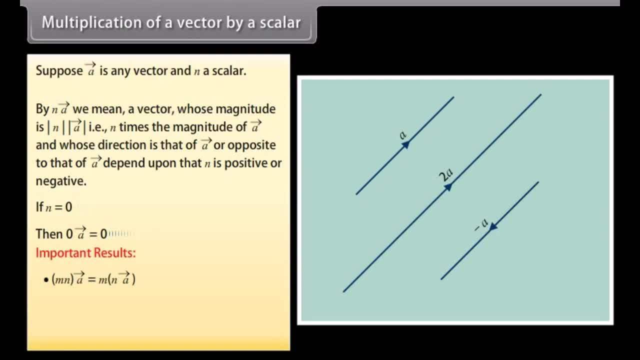 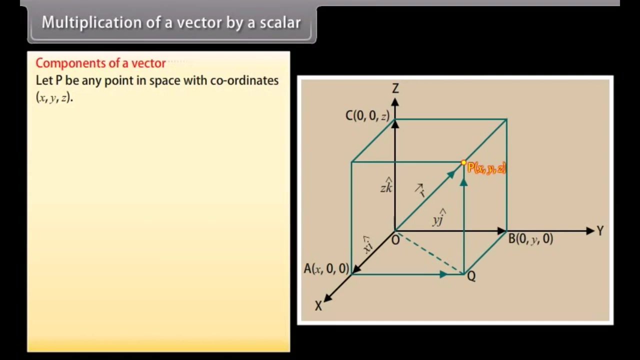 Mn vector A equals M into N vector A. N into vector A plus vector B equals N vector A plus N vector B. M plus N into vector A equals M into vector A plus N into vector A. Components of a vector. Let P be any point in space with coordinates x, y, z. 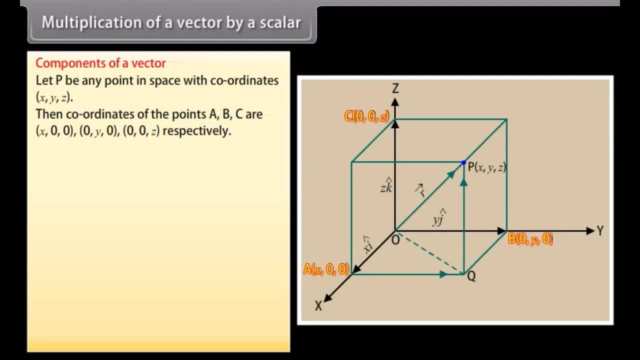 Then coordinates of the points A, B, C are x, 0, 0, y, 0, 0, 0, z Respectively. Suppose now that position vector of P is vector R, That is, vector OP equals vector R. Also, let cap I, cap J, cap K. 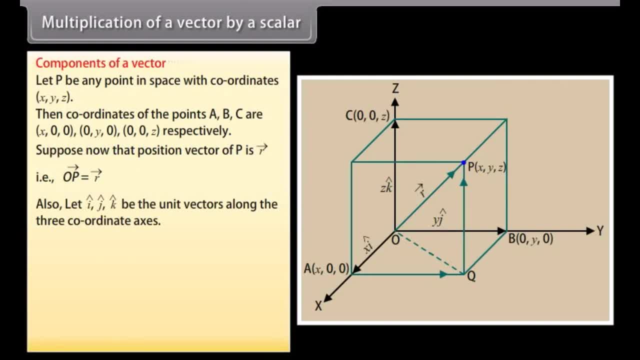 Be the unit vectors along the three coordinates axes. Now, OA equals x. It implies Vector OA is equal to x cap. I Note that x cap I is a vector whose magnitude is 1 into x equals x And whose direction is that of the x axis. And this is precisely the vector OA. 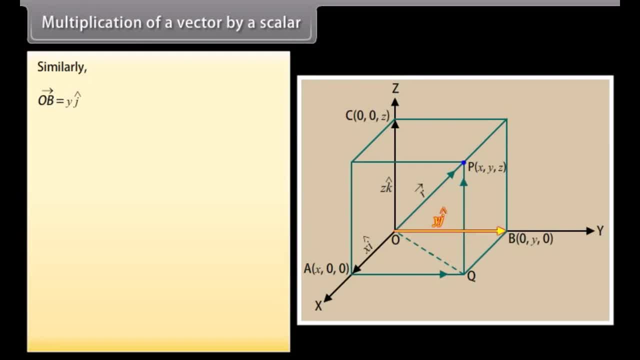 Similarly, Vector OB is equal to y cap J, Vector OC is equal to z cap K. From the triangle OPQ, Vector R equals vector OP. equals vector OQ plus vector QP equals vector OQ plus vector OC. Also, from the triangle OAQ, Vector OQ equals vector OA plus vector AQ equals vector OA plus vector OB. 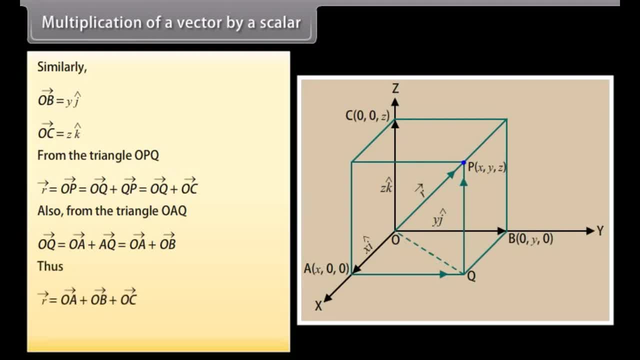 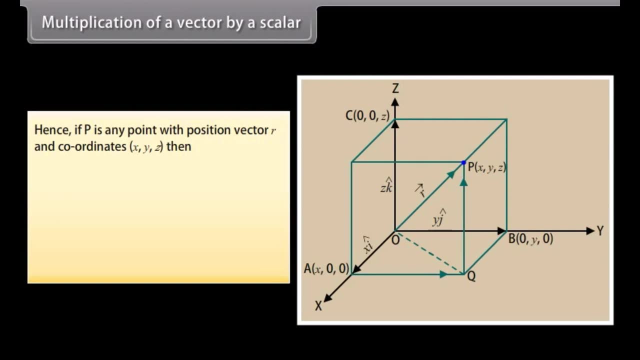 Thus Vector R equals vector OA plus vector OB plus vector OC, Vector R equals x cap I plus y cap J plus z cap K. Hence, If P is any point with position vector R And coordinates x, y, z, Then Vector R is equal to x cap I plus y cap J plus z cap K. 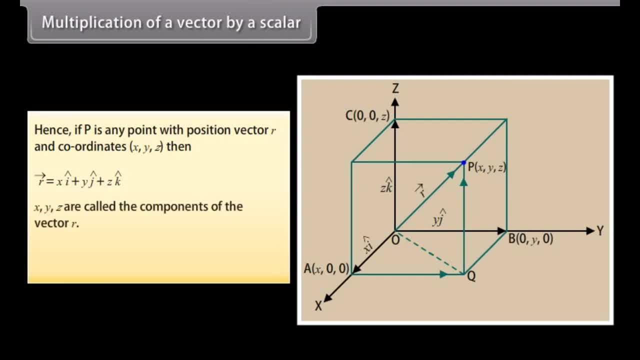 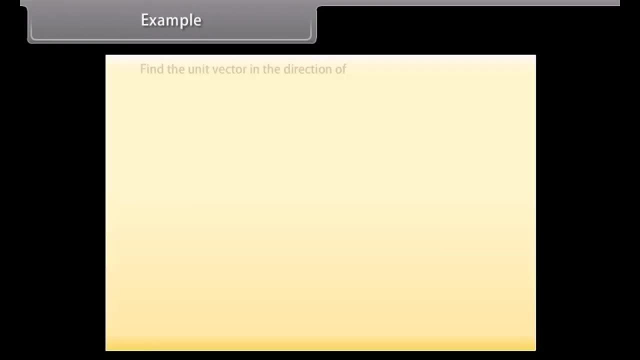 x, y, z are called the components of the vector. R Mode of vector is square root of x square plus y square plus z, square Example. Find: the unit vector in the direction of Vector A equals 4 cap I minus 8 cap J minus 7 cap K. 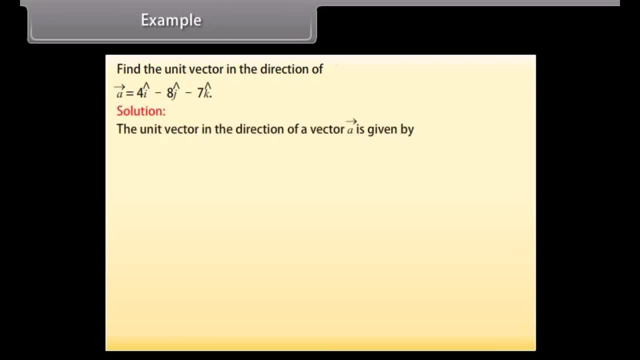 Solution: The unit vector in the direction of vector A is given by Cap A. equals vector A upon mode of vector A. Now, mode of vector A: equals Square root of 4 square plus minus 8 square plus minus 7 square. equals Square root of 16 plus 64 plus 49. equals square root of 129. equals 11.35. 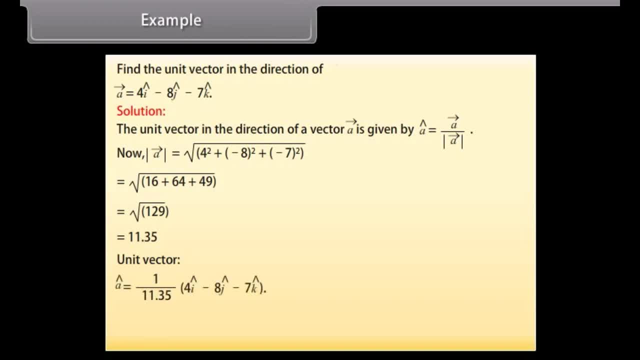 Unit vector is: Unit vector A equals 1 by 11.35 into 4 cap I minus 8 cap J minus 7 cap K: Unit vector A equals 4 cap I by 11.35 minus 8 cap J by 11.35. 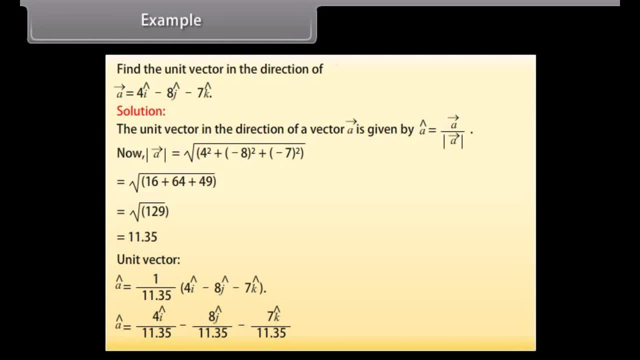 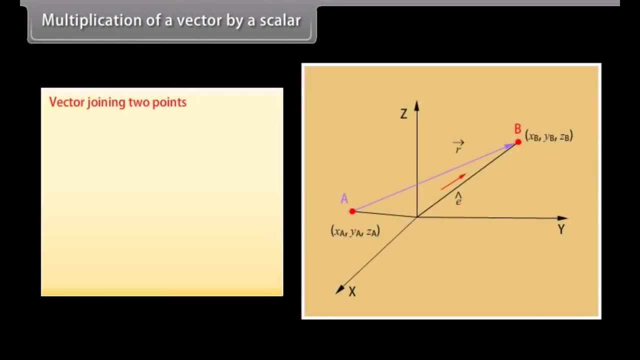 Unit. vector B equals 8 cap J minus 8 cap K by 7 cap J minus 7 cap K by 11.35. Solution: Multiplication of a vector by a scalar Vector joining two points. The vector connecting point A to point B is given by: 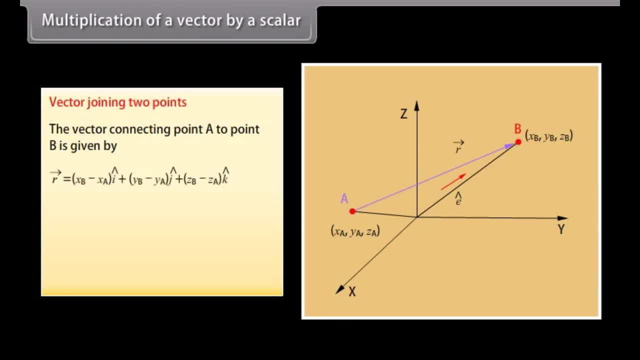 Solution: Vector R equals x b minus xA cap I plus y b minus y A cap J plus r b minus x A cap I plus r b minus y A cap J plus y B minus y A cap J plus y B minus y A cap and the end between points A and end to the end of the vector. including 2 points in the vector. 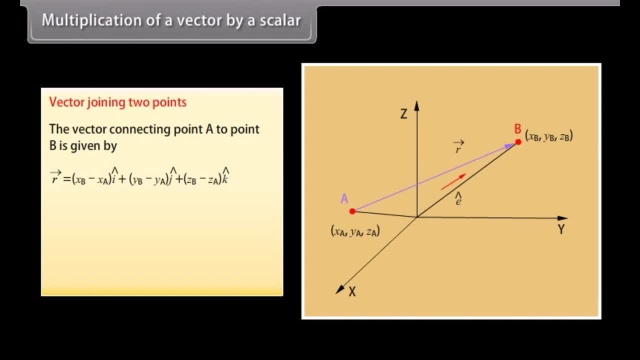 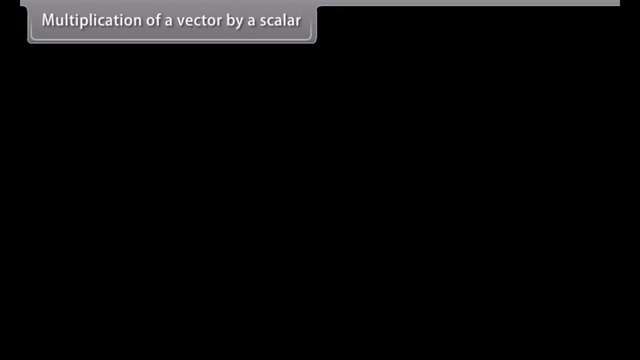 Solution: plus ZB minus ZA, cap K. The magnitude of the vector R is given by: magnitude of the vector R is square root of XB minus XA, whole square. plus YB minus YA, whole square. plus ZB minus ZA, whole square. Multiplication of a vector by a scalar. 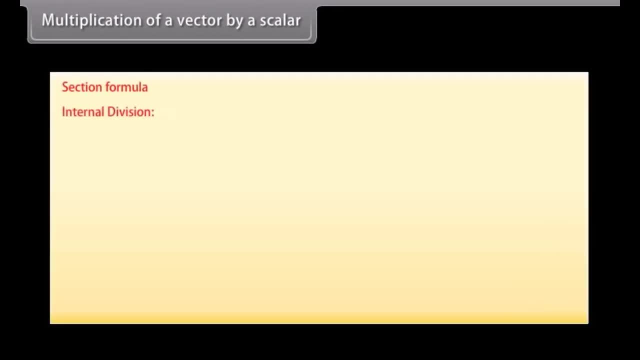 Section formula: Internal division. If vector A and vector B are the position vectors of two points, A and B, then the point C, which divides AB internally in the ratio M is to N, has the position vector. vector C equals M into vector B plus N, into vector A by M plus N. 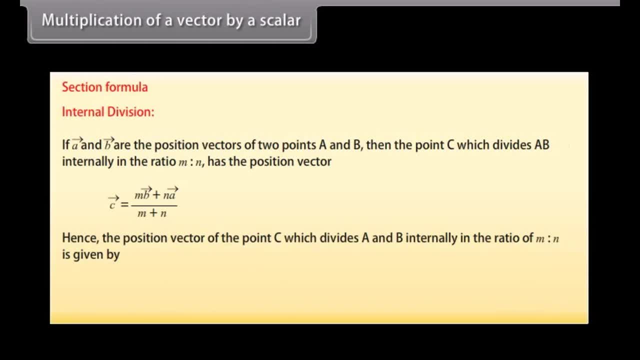 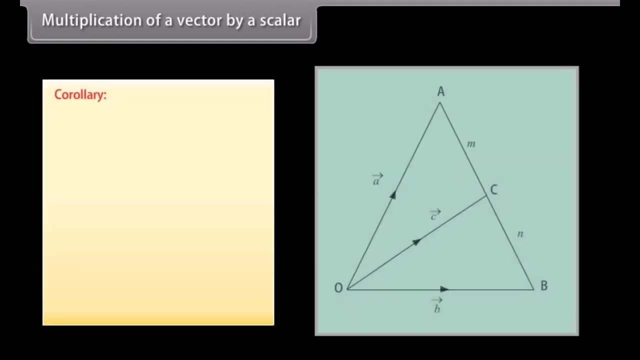 Hence the position vector of the point C, which divides A and B internally in the ratio of M is to N, is given by vector OC, equals M into vector B plus N, into vector A, by M plus N, Corollary, If C is the midpoint of AB. 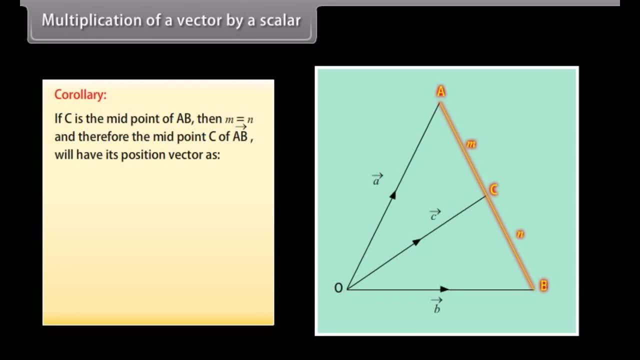 then M equals N and therefore the midpoint C of vector AB will have its position vector as given below. Vector OC equals vector A plus vector B by 2.. Vector OC equals vector A plus vector B by 2.. Vector OC equals vector OA plus vector OB by 2.. 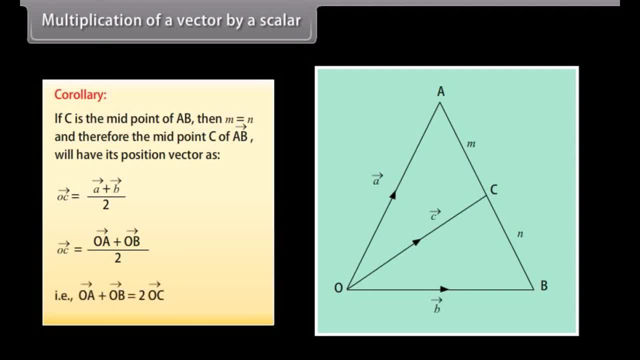 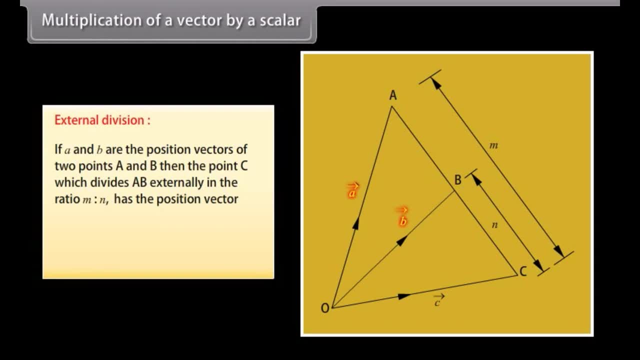 Vector OA plus vector OB equals 2 vector OC External division. If A and B are the position vectors of two points, A and B, then the point C, which divides AB externally in the ratio M is to N, has the position vector. vector C equals M into vector B. 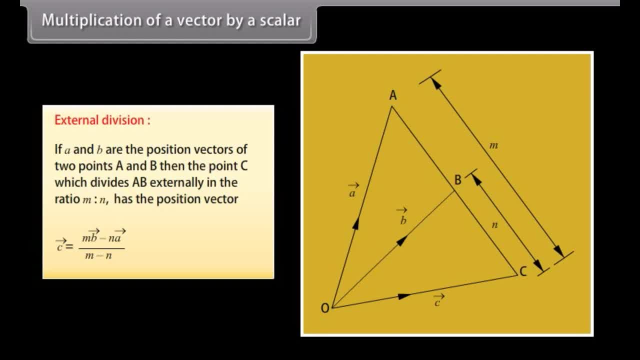 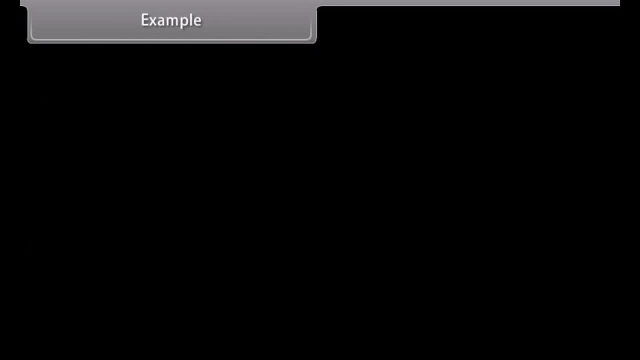 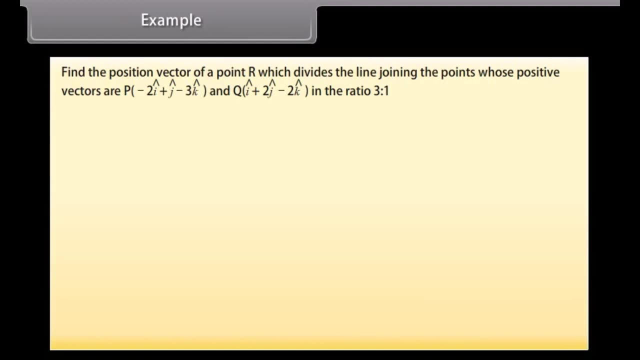 minus N into vector A by M minus N. Example: Find the position vector of a point R which divides the line joining the points whose positive vectors are P minus 2 cap I plus cap J minus 3 cap K and Q cap I plus 2 cap J minus 2 cap K. 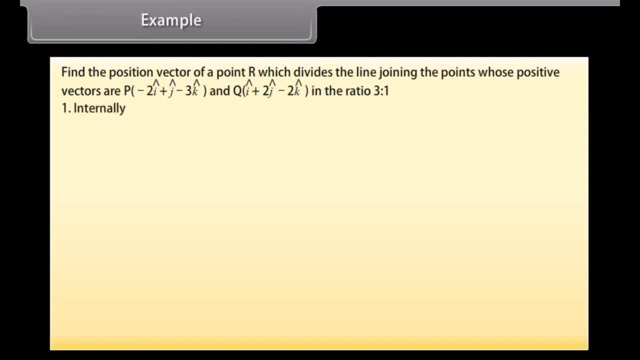 in the ratio 3 is to 1.. 1, internally, 2, externally. Solution: 1, internally. The position vector of point R, which divides the line joining the points P and Q in the ratio M, is to N. 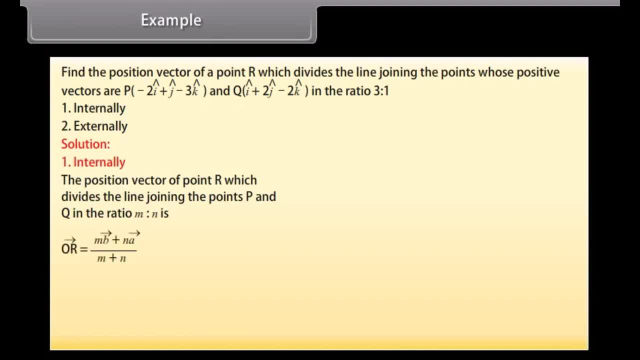 is vector OR equals M. vector B plus N, vector A by M plus N. Here M is equal to 3, N equals 1.. Vector A equals vector A plus vector B by M plus N, Or Vector B equals 2 cap I plus I plus. 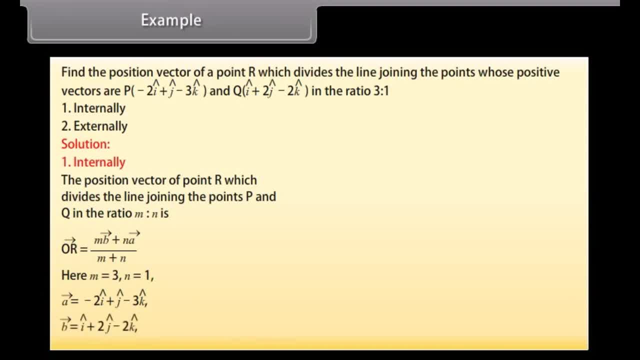 plus 3 cap J minus 3 cap K. Or vector B equals 2 cap I plus 2 cap J plus 2 cap K. Vector A equals vector C45, plus called R, or vector W equals 3 cap I plus I plus both I. 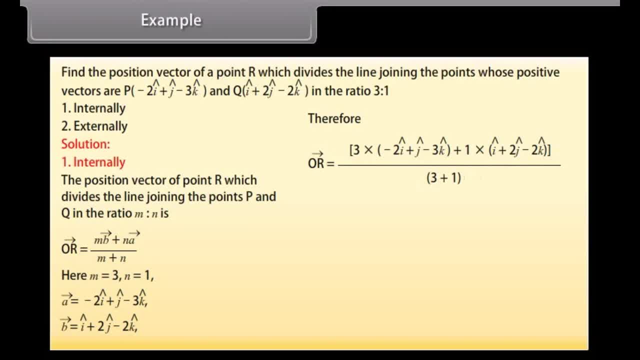 or vector C positive. third nature is X or vector O multiple of minus 3 sign. or vector O is equal to bottle leer or vector C inまた cue. or vector O is equal to brings or vector R by minus 2 cap into, or vector R over 1,. 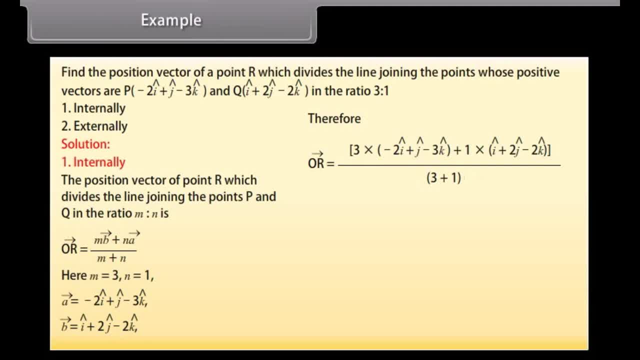 or vector O minus 3 cap I plus 3 cap K or vector O is equal to minus V by W. or vector O should be placed back, or vector Z or vector R would be placed back. We already know that 5 cap J minus 11 cap K by 4. 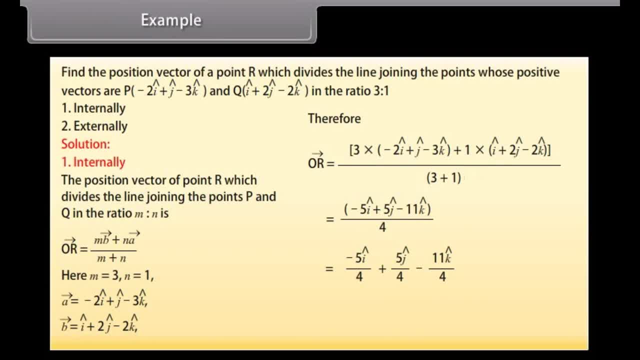 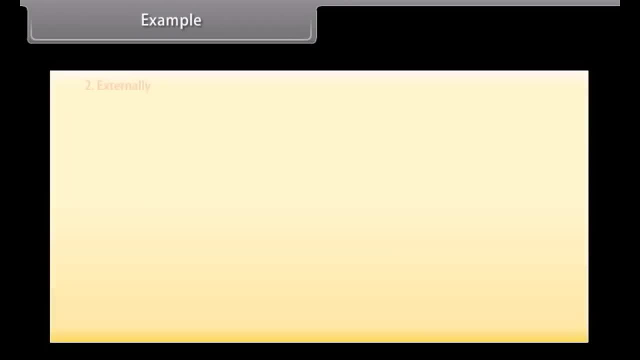 which is equal to minus 5 cap I by 4 plus 5 cap J by 4 minus 11 cap K by 4.. Externally, vector OR is equal to m. vector B minus n. vector A by m minus n. Therefore, vector OR is equal to. 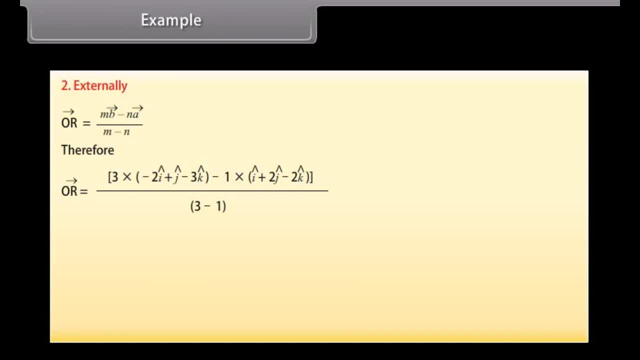 3 into minus 2 cap I plus cap J minus 3 cap K minus 1 into cap I plus 2 cap J minus 2 cap K. by 3 minus 1 equals minus 7 cap I plus cap J minus 7 cap K. 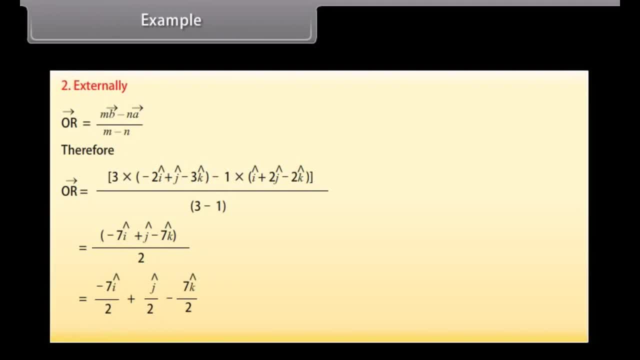 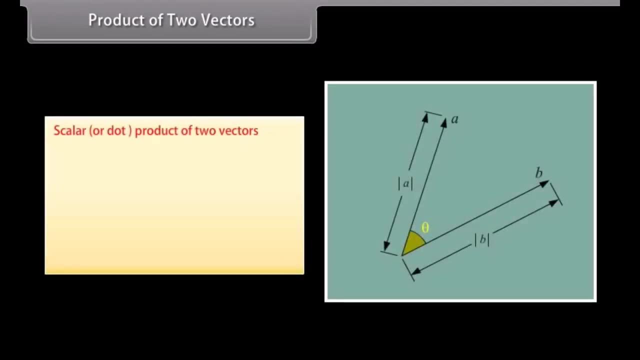 by 2 equals minus 7 cap I by 2, plus cap J by 2, minus 7 cap K by 2.. Plus product of two vectors: Scalar or dot, product of two vectors. The dot product of two vectors, A and B, is: 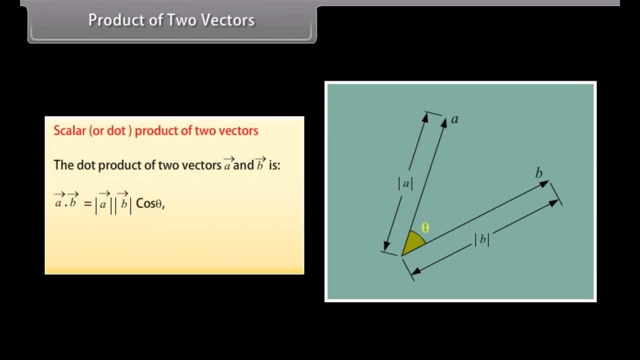 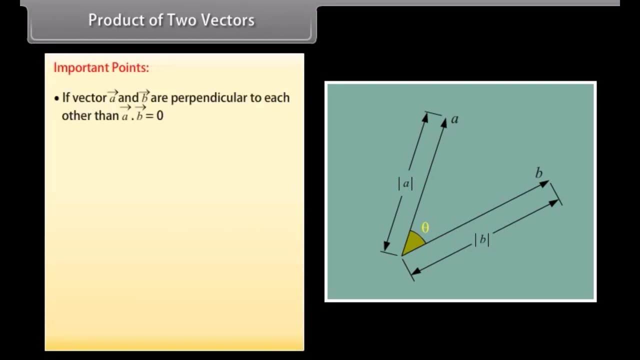 magnitude of A times the magnitude of B. then multiply the cosine of the angle between A and B, where theta is the angle between vector A and B. Important points: If vector A and B are perpendicular to each other, then dot product of vector A and B. 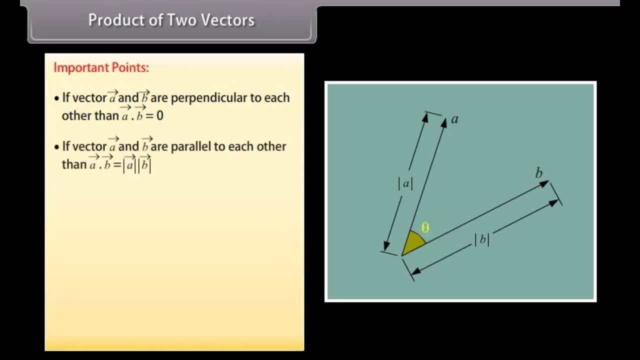 is 0.. If vector A and B are parallel to each other, then dot product of vector A and B is magnitude of vector A into magnitude of vector B. The unit vectors cap I, cap J and cap K are perpendicular to each other. 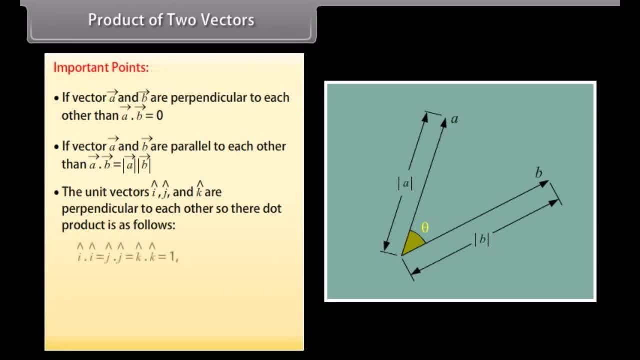 So their dot product is as follows: cap I dot cap I equals cap J. dot cap J equals cap K. dot cap K equals 1.. cap I dot cap J equals cap J. dot cap K equals cap K. dot cap I equals 0.. 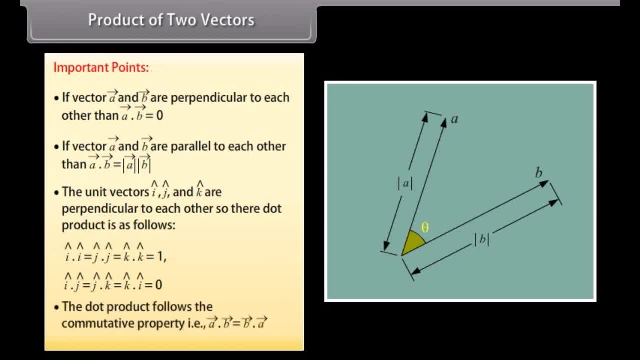 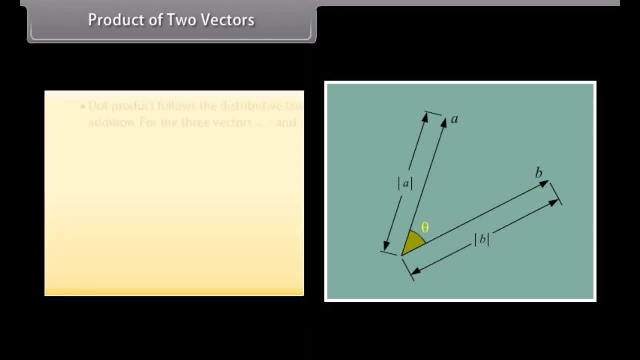 The dot product follows the commutative property, That is, dot product of vector A and B is equal to dot product of vector B and A. Dot product follows the distributive law of addition for the three vectors A, B and C. Dot product of vector A and vector B. 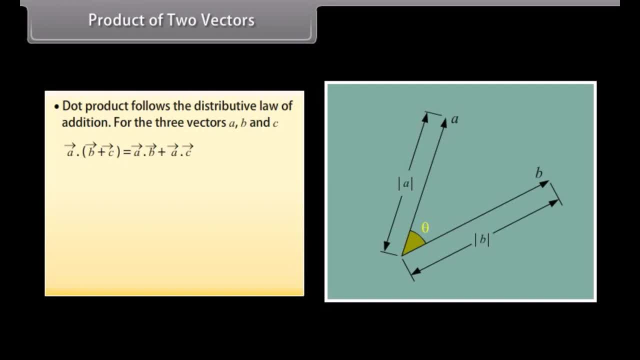 plus vector C is equal to dot product of vector A and B plus dot product of vector A and C. If vector A is equal to A1 cap I plus A2 cap J plus A3 cap K, vector B equals B1 cap I plus B2 cap J. 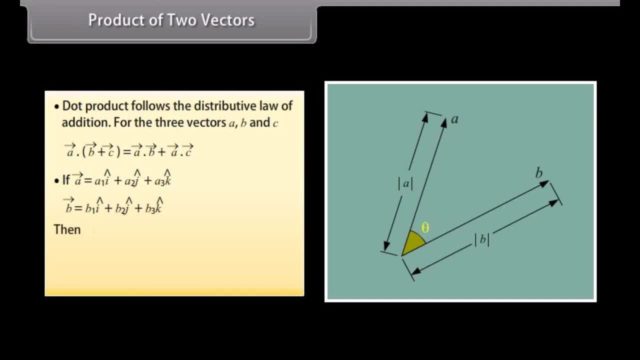 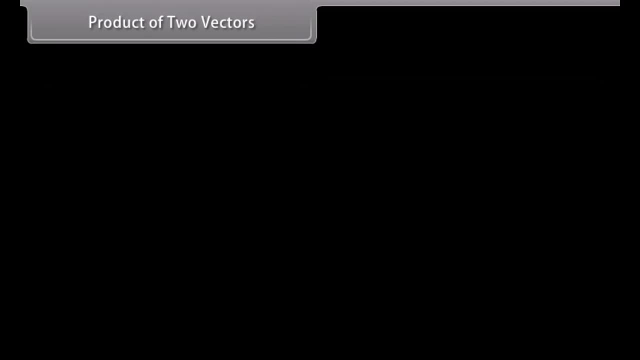 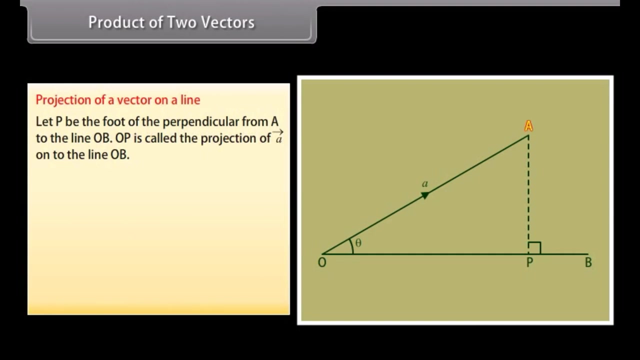 plus B3, cap K then dot. product of vector A and B equals A1, B1 plus A2, B2 plus A3, B3 et al. product of two vectors. Projection of a vector on a line. Let P be the foot of the perpendicular from A. 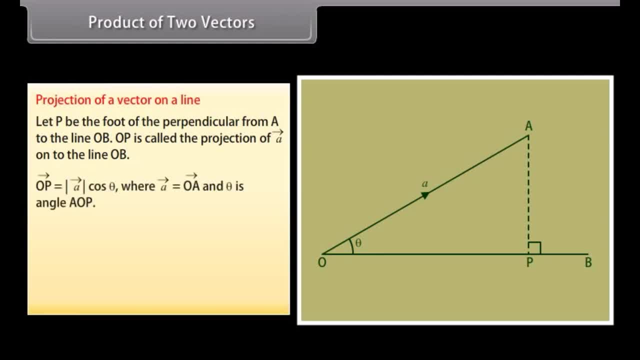 to the line O B. O B is called the projection of vector A on the line O B. Vector O B is equal to magnitude of vector A into cos theta, where vector A is equal to vector OA and Peter's angle, aOP. Information 4 & Як in English sehen hier. 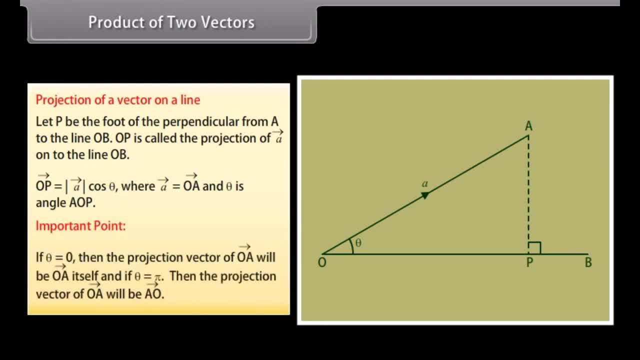 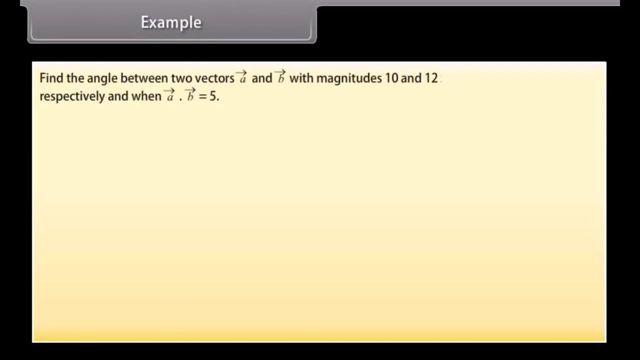 Important point point: If theta is equal to zero, then the projection vector of OA will be vector OA itself, and if theta is equal to pi, then the projection vector of OA will be vector AO. Example: Find the angle between two vectors A and B, with magnitudes 10 and 12 respectively. 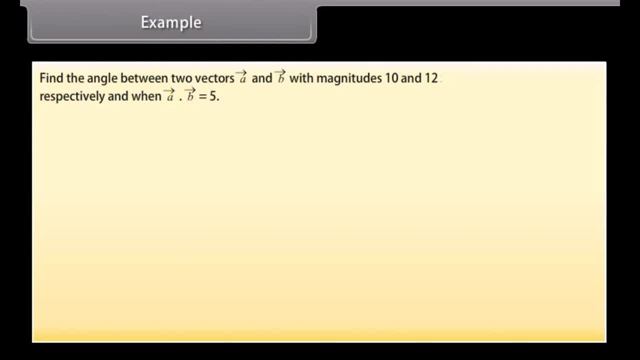 and when: dot product of vectors A and B is equal to 5. Solution: The dot product of vector A and B. magnitude of A and B is equal to 5. Solution: The dot product of vector A and B: magnitude of A times the magnitude of B. then multiply the cosine of the angle between A and B. 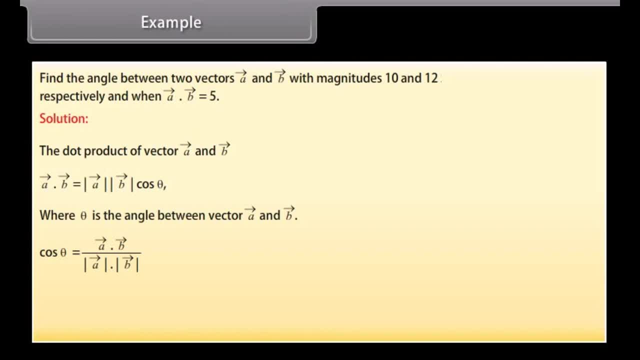 Cos. theta is equal to dot product of vector A and B by magnitude of vector A into magnitude of vector B. Theta equals cos inverse dot product of vector A and B by magnitude of vector A into magnitude of vector B. Theta equals cos inverse 5 by 10 into 12.. Theta equals cos inverse 5 by: 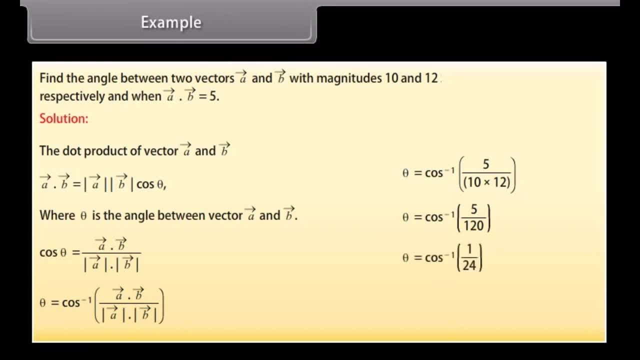 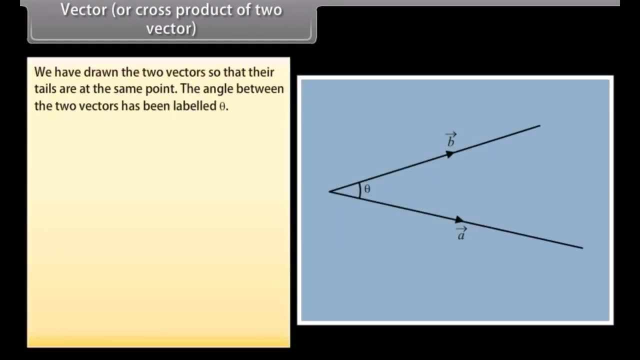 120.. Theta equals cos inverse 1 by 24.. Theta equals cos inverse 0.04167.. Theta is equal to 87.61 degree Vector, a cross product of two vectors. We have drawn the two vectors so that their tails are at. 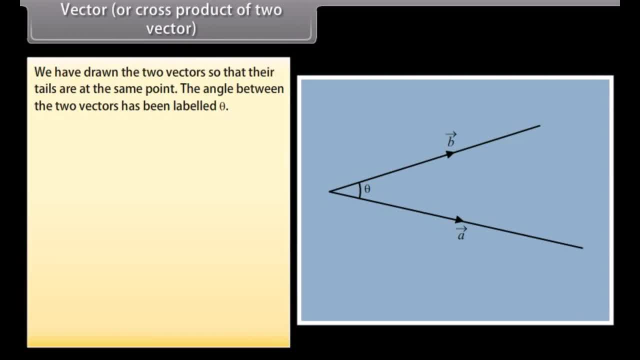 the same point. The angle between the two vectors has been labeled theta. When we find a vector product, the result is a vector. First we define the modulus or magnitude of this vector as magnitude of vector A, Vector A into magnitude of vector B, into sine of theta. To obtain a vector, we need to specify a. 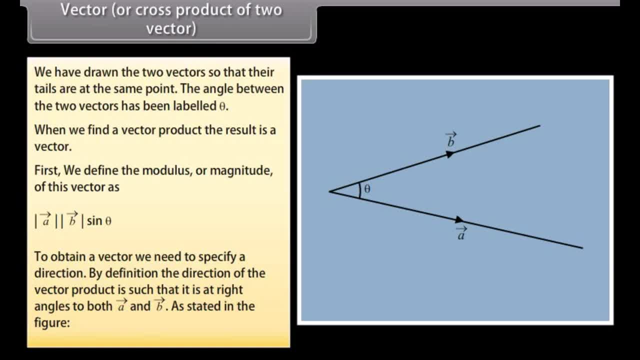 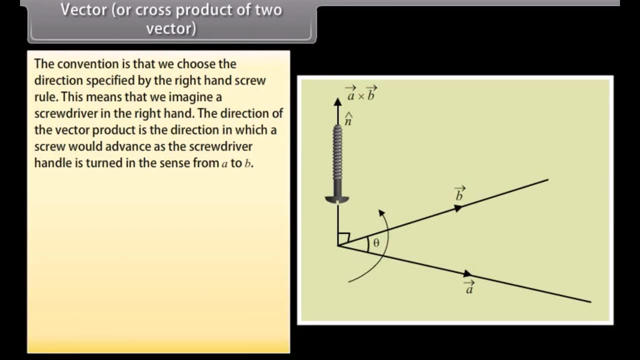 direction. By definition, the direction of the vector product is such that it is at right angles to both vectors A and B, As stated in the figure. the convention is that we choose the direction specified by the right hand screw rule. This means that we imagine a screwdriver in the right hand. 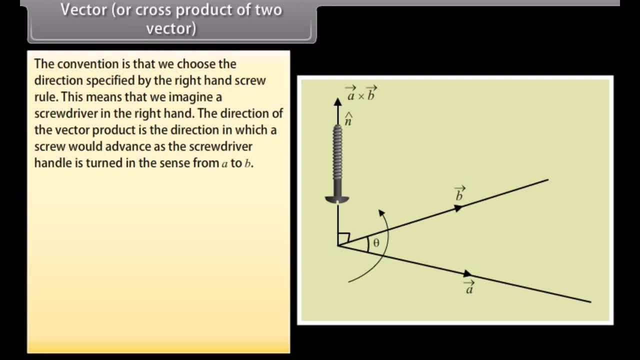 The direction of the vector product is the direction in which a screw would advance as the screwdriver handle is turned, in the sense from A to B. The vector product of A and B is defined to be Vector A cross vector B equals magnitude of vector A into magnitude of vector B, into sine of theta. 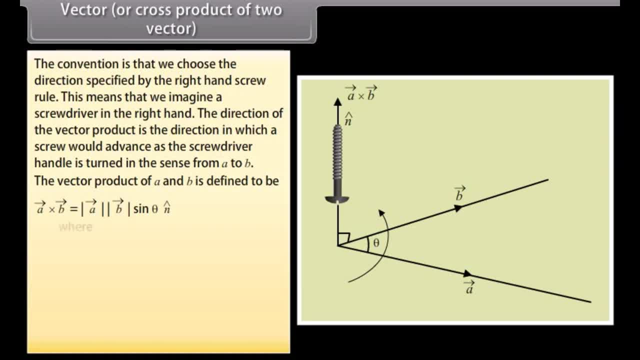 in the direction of Ncap, Where magnitude of vector A is the modulus of magnitude of A, Magnitude of vector B is the modulus of the main vector function of root number 1, and the вдруг and end of regularness bookstore. 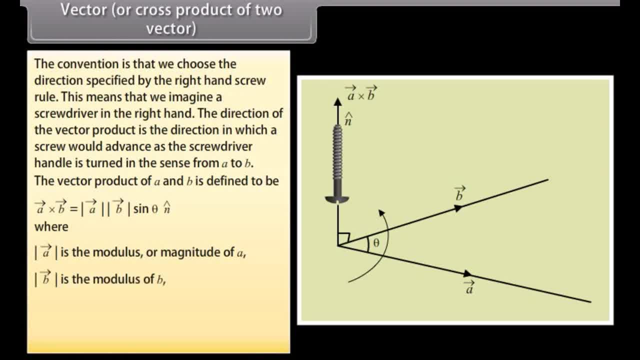 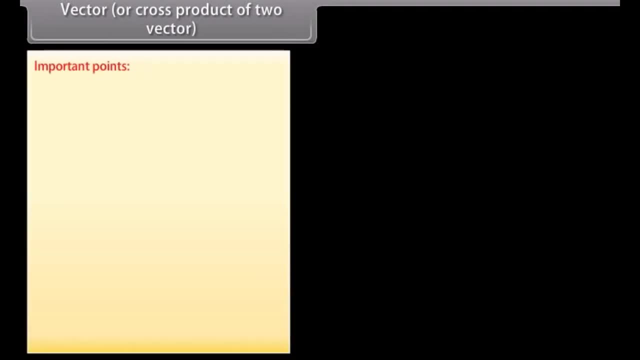 Magnitude of vector B is the modulus of B, Theta is the angle between vector A and B and cap N is a unit vector perpendicular to both vector A and B, in a sense defined by the right-hand screw rule. Important points: Vector product of unit vectors which are perpendicular to each other is as follows: 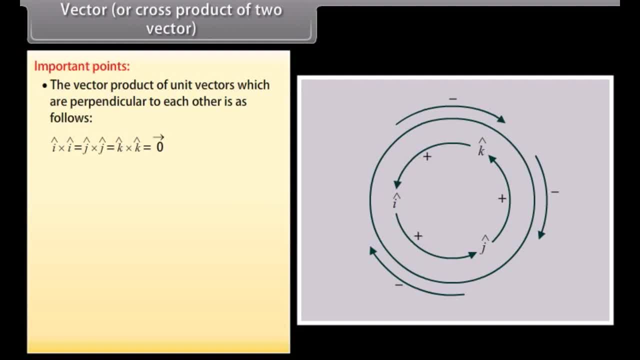 Cap I cross cap I equals cap J. cross cap J Equals cap K. cross cap K equals vector 0.. Cap I cross cap J equals cap K. Cap J cross cap K equals cap I. Cap K cross cap I equals cap J. Cap J cross cap I equals minus cap K. 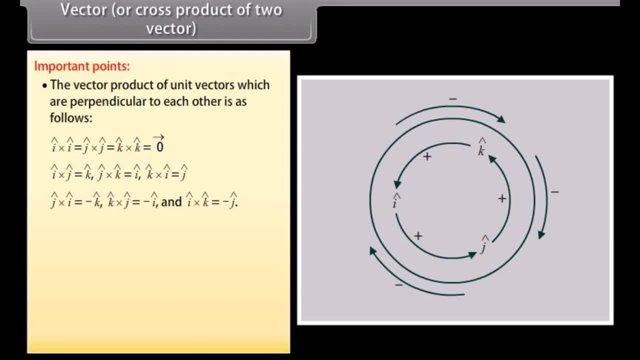 Cap K cross cap J equals minus cap I. Cap I cross cap K equals minus cap J. If vectors A and B represent the adjacent sides, then its area is given by magnitude of vector product of vectors A and B. If vectors A, B and C are three vectors, 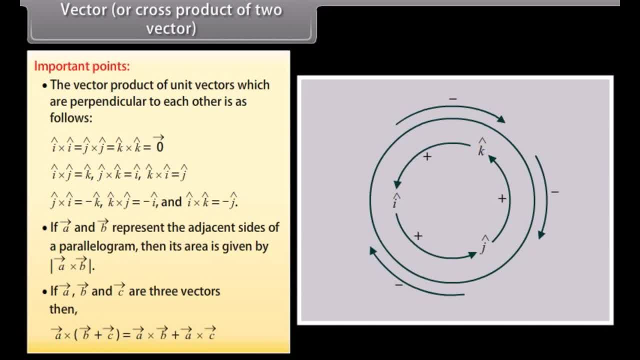 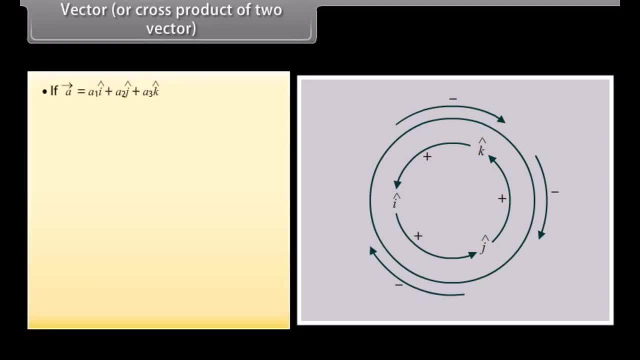 then vector A cross vector B plus vector C equals vector A cross vector B plus vector A cross vector C. If vector A is equal to A1 cap I plus A2 cap J plus A3 cap K. vector B equals B1 cap I plus A2 cap J plus A3 cap K. 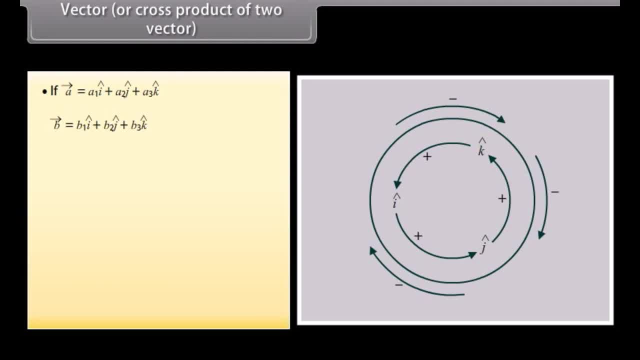 If vector A and B are equal to A1, cap I plus B2, cap J plus B3, cap K, then vector product of A and B is equal to determinant of row-wise: first row, cap I, cap J, cap K. second row, A1, A2, A3,. third row, B1, B2, B3.. 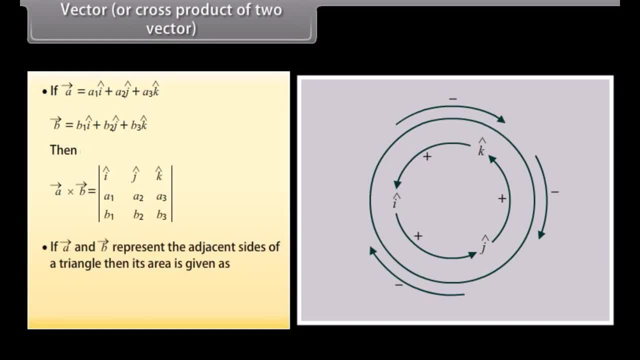 If vectors A and B represent the adjacent sides of a triangle, then its area is given as 1 upon 2 into magnitude of vector product of A and B. If vectors A and B are equal to, A and B represent the adjacent sides of a triangle. 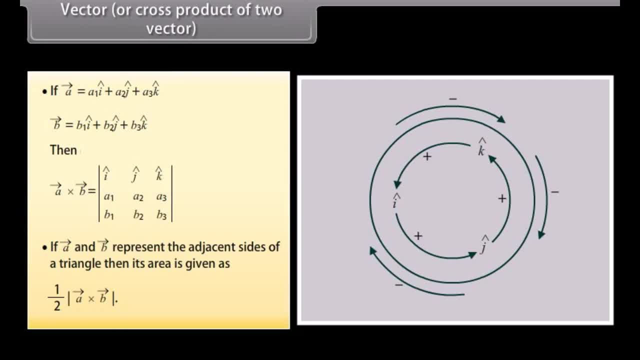 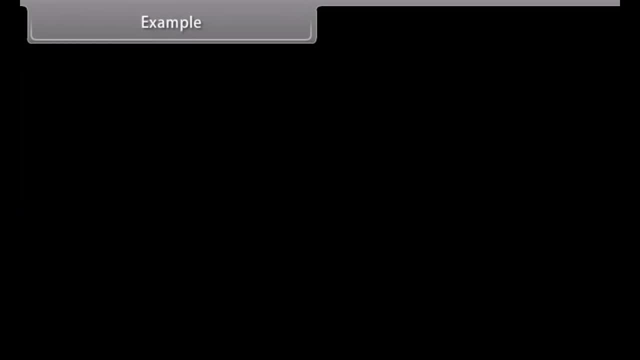 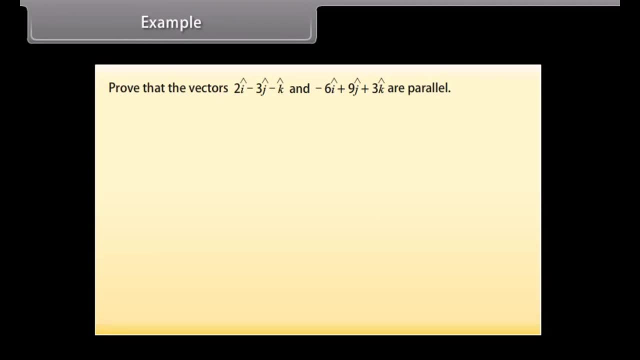 to product of A and B. Example Prove that the vectors 2 cap i minus 3 cap j minus cap k and minus 6 cap i plus 9 cap j plus 3 cap k are parallel Solution: The given vectors will be parallel if their cross product is 0. 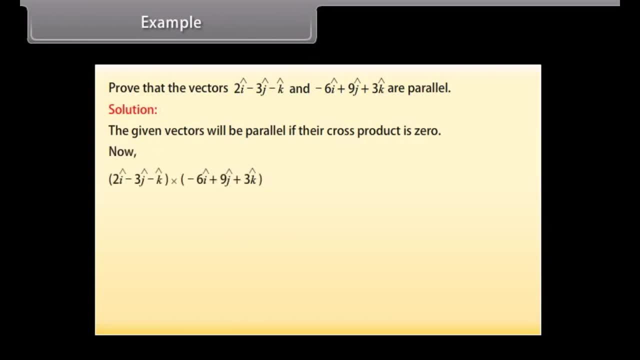 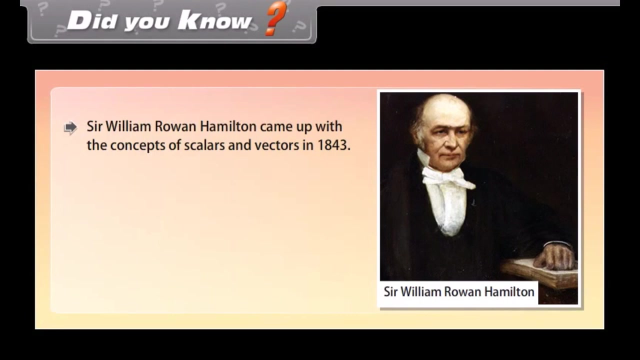 Now 18 cap k equals 0. Hence proved. Did you know? Sir William Rowan Hamilton came up with the concepts of scalars and vectors in 1843.. William Rowan Hamilton's scientific career included the study of optics. 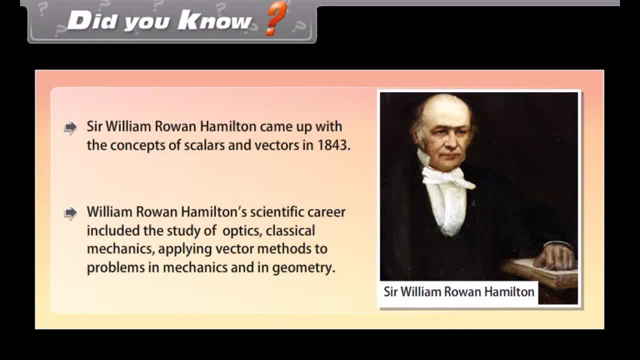 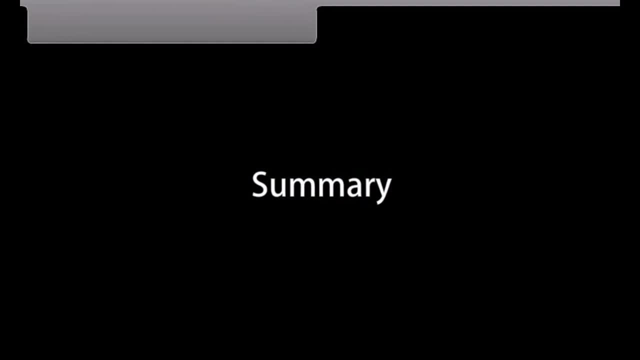 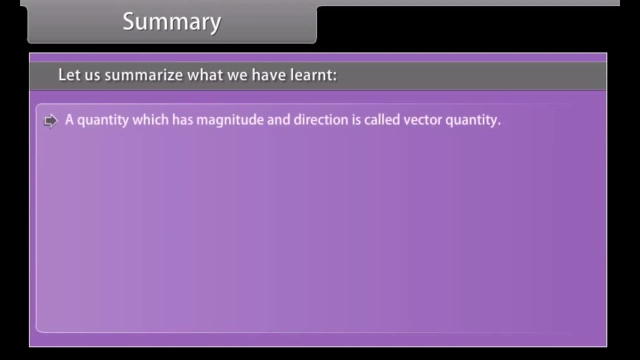 classical mechanics, applying vector methods to problems in mechanics and in geometry. Summary: Let us summarize what we have learned. A quantity which has magnitude and direction is called vector quantity. Let O be a fixed point in space called the origin of reference, and P be any point whose coordinates are x, y, z. 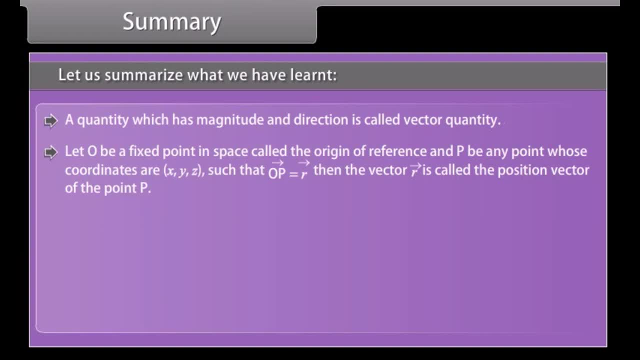 As such that vector O, P is equal to vector R, then the vector R is called the position vector of the point P Direction cosines are: L equals cos alpha, M equals cos beta, N equals cos gamma, And they are connected by the formula L square plus M square plus N square equals 1.. 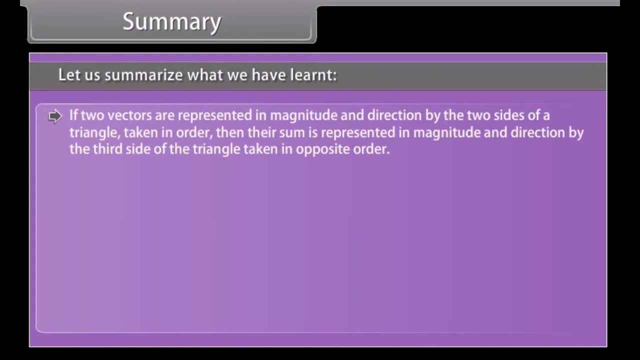 If two vectors are represented in magnitude and direction by the two sides of a triangle- sides of a triangle taken in order- then their sum is represented in magnitude and direction by the third side of the triangle, taken in opposite order. If two vectors are represented in magnitude and direction by two adjacent sides of a parallelogram. 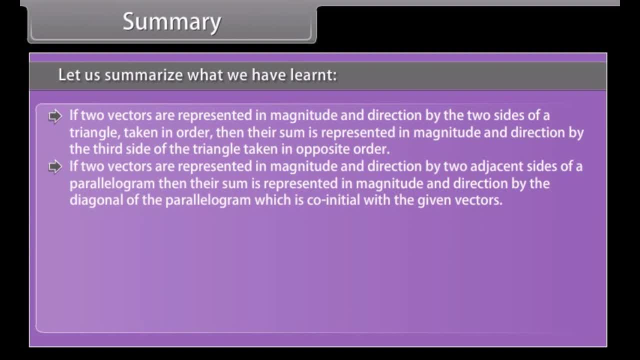 then their sum is represented in magnitude and direction by the diagonal of the parallelogram which is co-initial with the given vectors: mn vector a equals m into n vector a. n into vector a plus vector b equals n vector a plus n vector b. 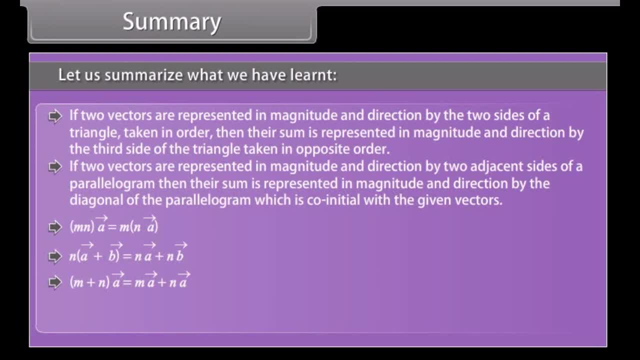 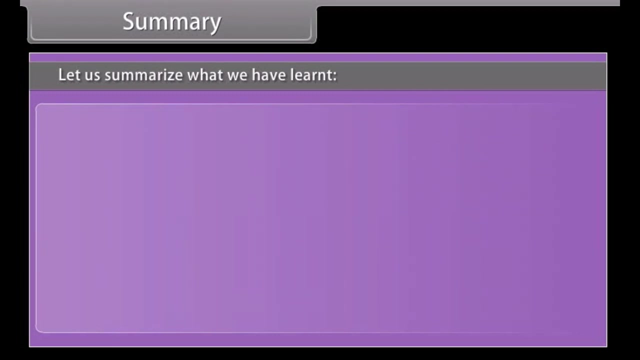 m plus n into vector a equals m into vector a plus n into vector a. The position vector can be represented as: vector r equals x cap i plus y cap j plus z cap k. If vector r is connecting two points- A, xA, yA, zA and B, xB, yB, zB- then vector r is: 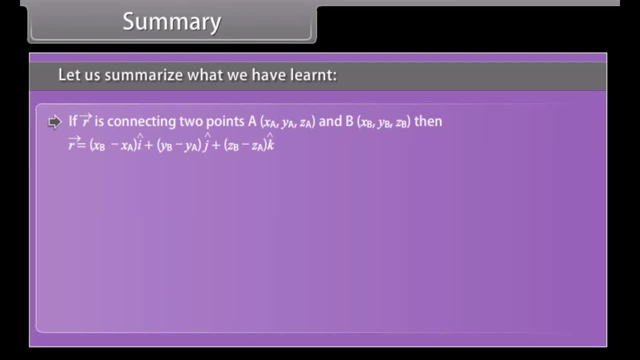 equal to xB minus xA cap i plus yB minus yA cap j plus zB minus zA cap k. If vector r is connecting two points, A and xB, yB, yA, cap x and zB means n компense. 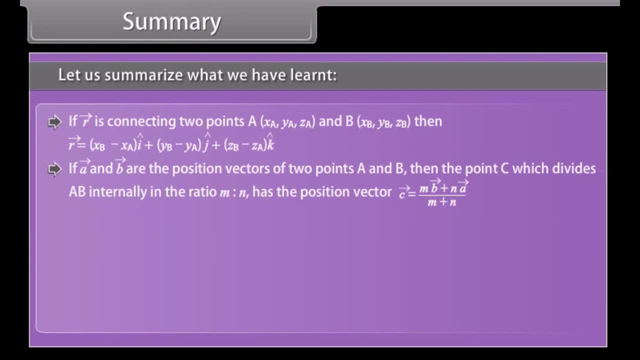 gigabytes of zA cap, Then vector r is rather exact. If vector r is between two points, A and xB q cap is separated away, Then vector r is connected to zB by xB and is the position of xB. 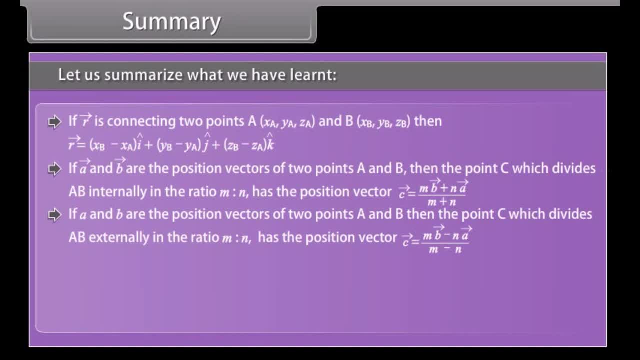 If vector r is interconnected by xB and yA as the position, then vector r is more specific detail. cum É es con helplessreath. m. into vector b minus n. into vector a by m minus n. The dot product of two vectors, a and b, is: